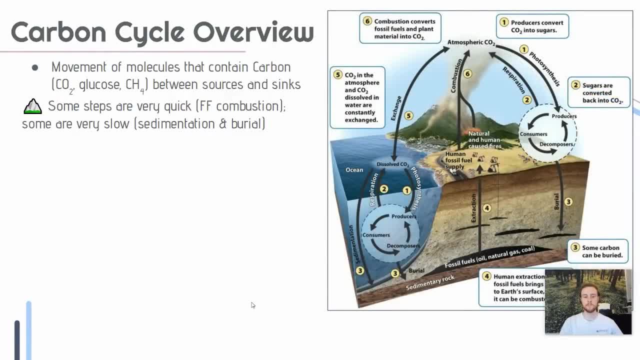 this diagram here. Imagine the shells of organic organisms or dead algae floating to the bottom of this ocean, So that's called sedimentation. And then, as they're compressed and buried into sedimentary rock or into fossil fuels, they're going to decompose into fossil fuels. So that's. 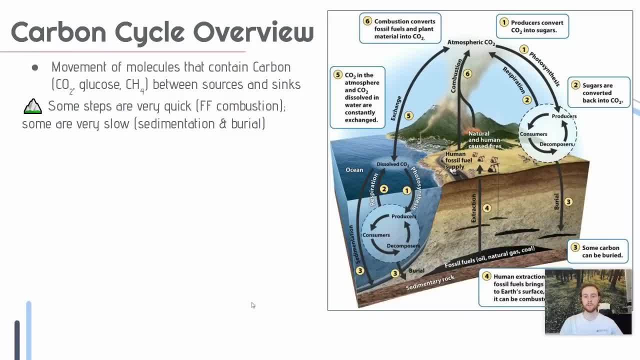 a really, really long process. Now, on the other hand, if we look at step four, the extraction, it's really really quick to dig up carbon and combust it, And that returns carbon to the atmosphere in the form of CO2.. So that's going to lead to an imbalance in the reservoirs that 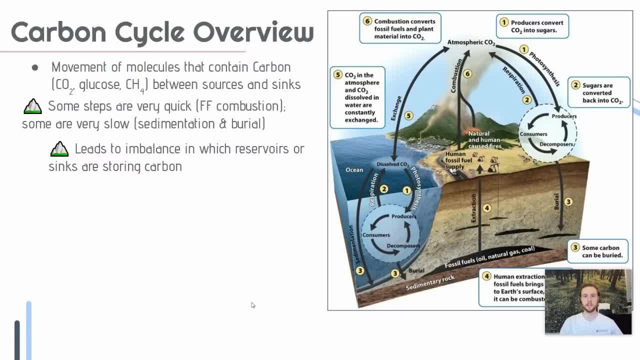 are storing carbon, Because digging up fossil fuels and combusting them releases carbon to the atmosphere far, far, far faster than it's removed through sedimentation and burial, leads to an imbalance and an increase in carbon dioxide in the atmosphere. Now, this is a problem because the atmosphere is a key reservoir of carbon, But as the level of 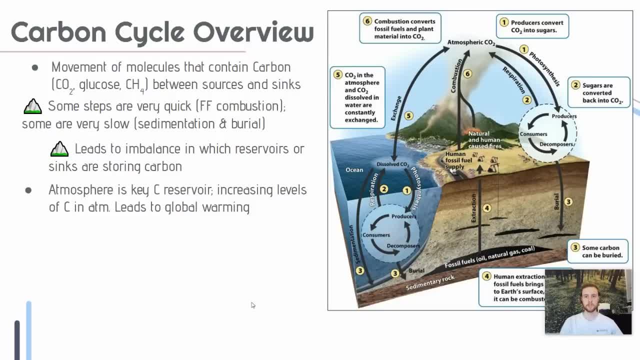 carbon dioxide in the atmosphere increases, so does the global temperature. So if you've heard of global warming or climate change, this is occurring because humans are increasing the concentration of carbon dioxide in the atmosphere, primarily by digging up these fossil fuels and burning them. So if we talk about carbon sinks, these are carbon reservoirs that are storing more. 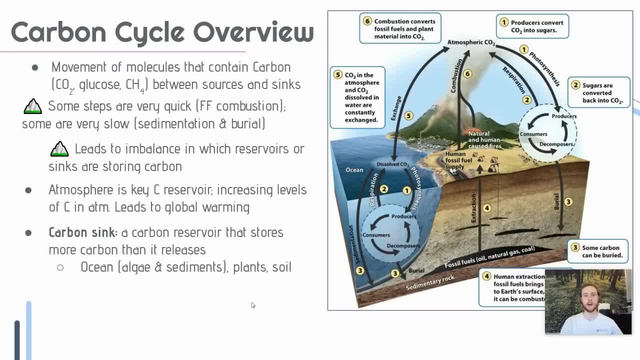 carbon than they release, So we can think of them as taking up fossil fuels and burning them. They're taking carbon out of the atmosphere so they can mitigate or reduce the effects of climate change. In the ocean, these are things like algae, which take in carbon dioxide through photosynthesis. 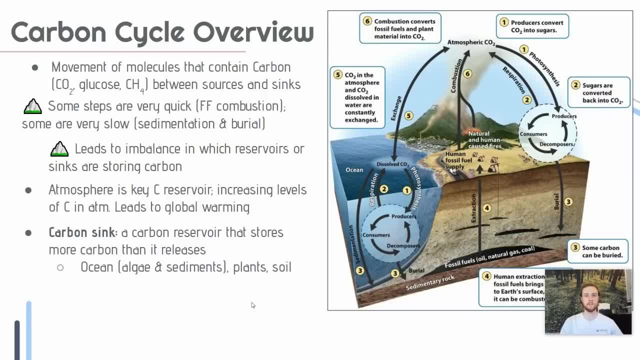 and sediments which store little bits of carbon in organic matter at the bottom of the ocean. And then on land we have plants which also do photosynthesis and store carbon in their tissues, either in glucose or in other structural compounds, And we also have the soil. 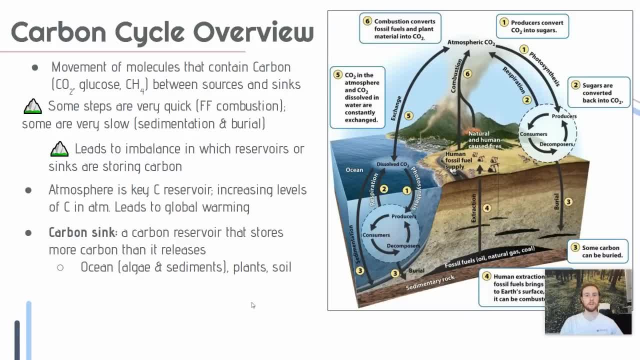 which can store carbon, as organisms die and decompose and their carbon is added to the soil. Carbon sources, on the other hand, are processes that release more carbon than they store, So this is going to increase the concentration of carbon dioxide in the atmosphere. Some of those are fossil fuel combustion, So this is oil, coal and natural 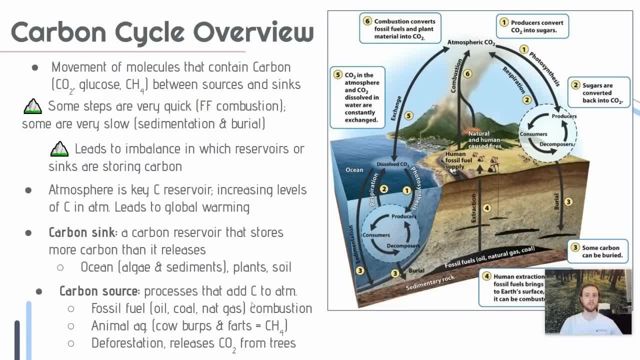 gas. We also have animal agriculture. Animal agriculture releases a lot of methane because the cows primarily, as well as other organisms that are grown for human food, are going to release a lot of methane through both their burps and their farts, And methane is a greenhouse gas. 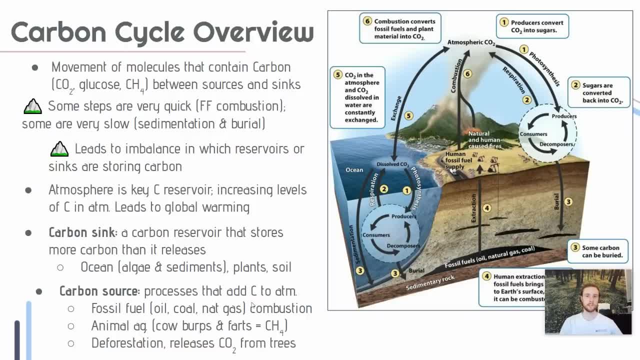 so that's also going to contribute to climate change. Then, finally, we have deforestation. So when we cut down trees for logging or just to clear land for agriculture, the carbon dioxide that they stored is released into the atmosphere and they don't go on storing more carbon dioxide, And so all of those are what we call carbon. 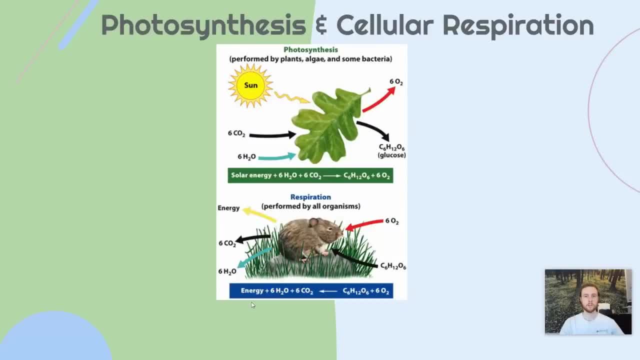 sources, which adds carbon to the atmosphere. Now we'll talk about photosynthesis and cellular respiration. So photosynthesis, of course, is carried out by plants, algae and phytoplankton. It's a process where remove carbon dioxide from the atmosphere and convert it to glucose. Now that glucose is an 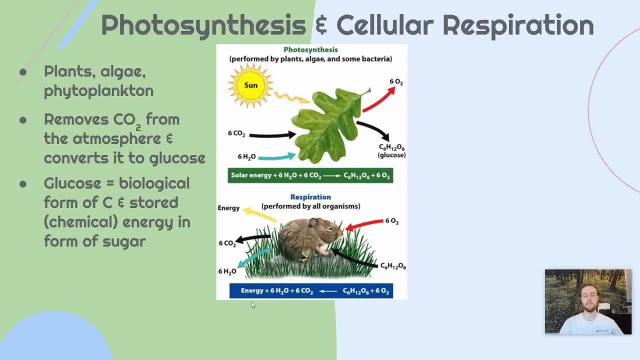 organic molecule, meaning it is created by a living thing, And it's a biological form of carbon And it's a storage molecule which stores energy that can be used later in the form of a sugar. Now this is a CO2 or a carbon sink, because it's going to remove carbon from the atmosphere in increasing 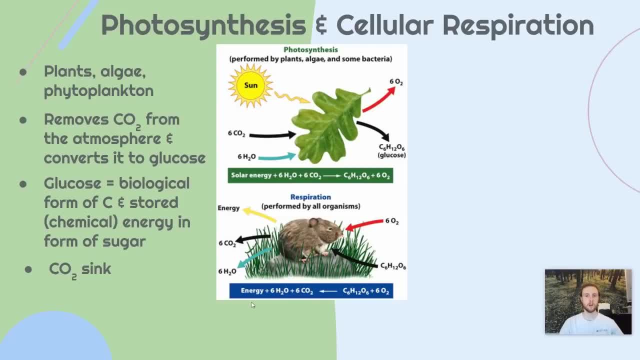 amounts. So as trees get taller, they're incorporating more and more carbon into their bark, into their roots, into their other structures. So again, you can think of those trees as just continually pulling CO2 out of the atmosphere- a carbon sink. Next we'll talk about 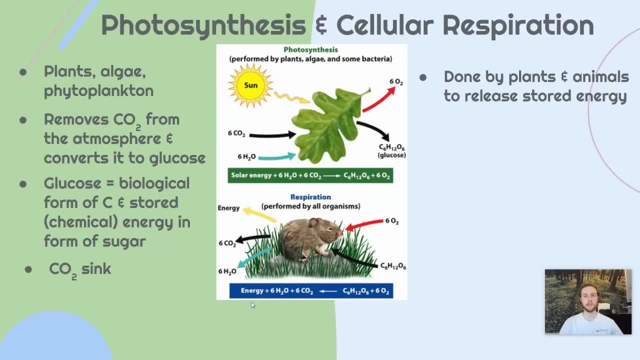 cellular respiration, So this is something that all living things do. One common misconception is that it's only animals. Another misconception is that it's just breathing. Breathing is just the act of pulling in air into your lungs, And that's not the same thing as respiration. 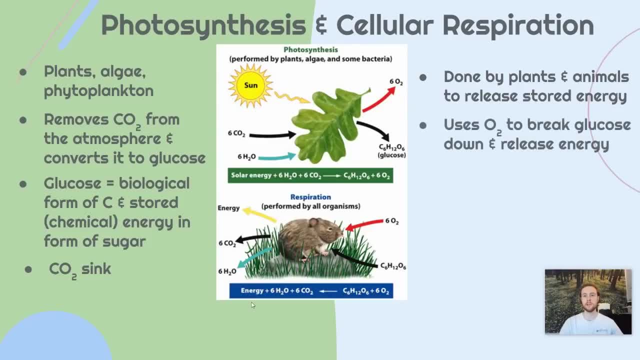 Cellular respiration is a process where organisms actually use up oxygen that they breathe in, And that's the act of pulling in air into your lungs, And that's not the same thing as breathing, And that's not the same thing as respiration. Cellular respiration is a process where 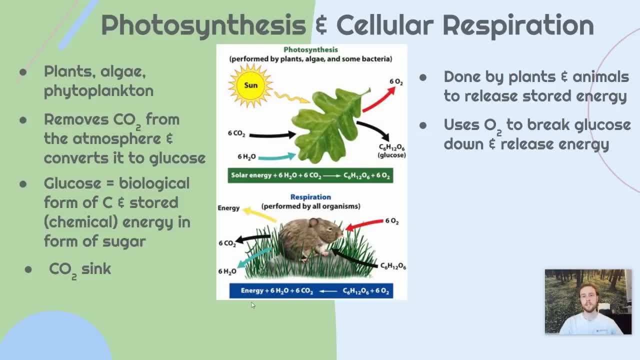 organisms actually use up oxygen that they breathe in to their lungs or take into their body in some other way, And they break down glucose to release energy. Now that energy could fuel their movement, It could fuel their growth, But that's the key of cellular respiration. You're. 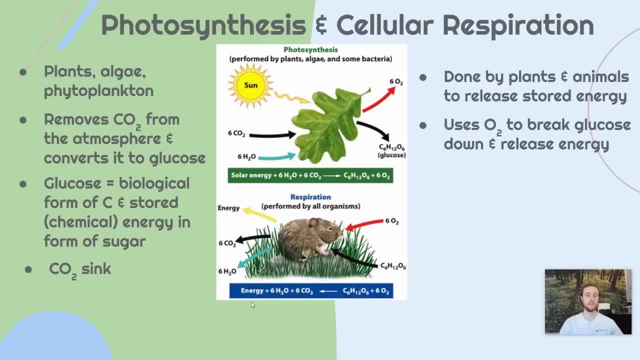 breaking glucose which, remember, has that carbon from the atmosphere to release energy, Because this process releases carbon dioxide in the atmosphere. we call it a carbon source. But it's very important to understand that both of these processes happen very quickly And both of these 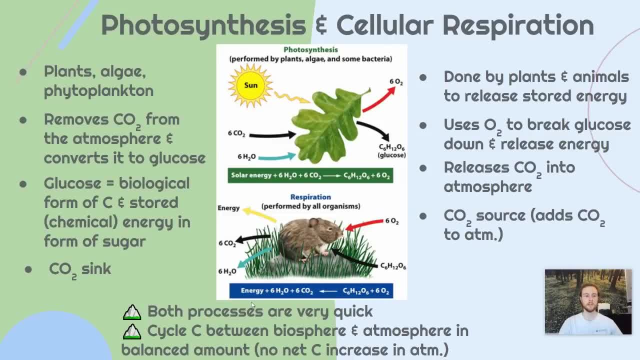 processes balance each other out. So if you look at the equation, in the top equation we have photosynthesis, releasing oxygen and producing glucose. And then if we look down at the bottom, for respiration organisms are going to take in oxygen and glucose, They're going to give off CO2,. 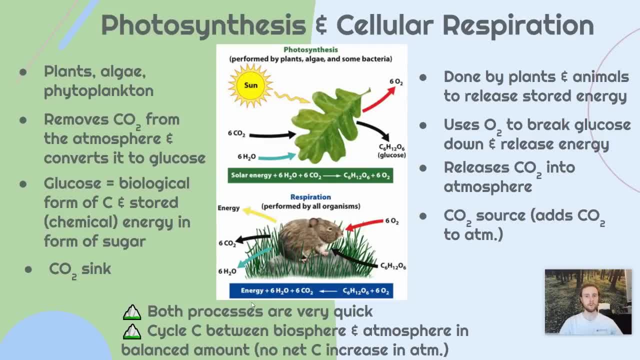 which plants then take back in to create glucose with. So these processes balance each other out And we call this no net increase in atmospheric carbon, because the carbon that's being produced by animals through respiration is taken up by plants to produce. 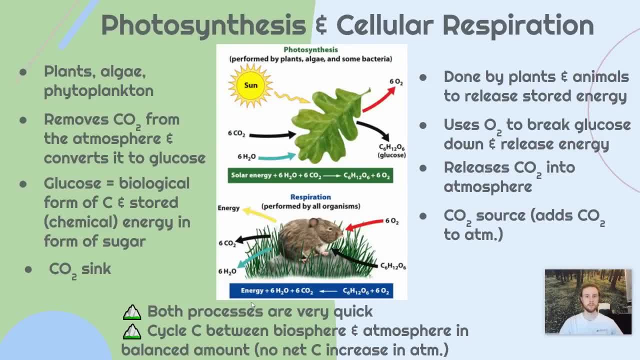 glucose. So think of these as a short-term cycle where the carbon is just kind of looping back and forth between plants and animals. We're not really increasing the net amount of carbon dioxide in the atmosphere because these processes are relatively balanced. Next we'll talk about how carbon cycles. 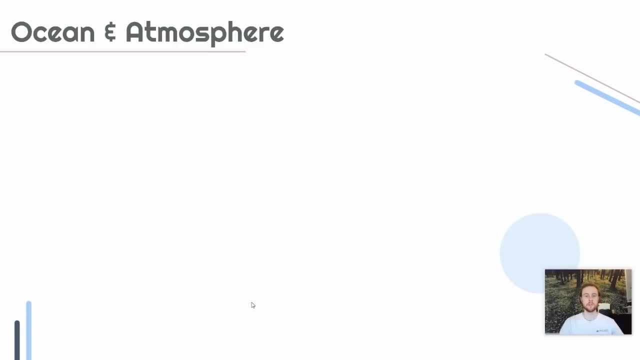 back and forth between the ocean and the atmosphere. So direct exchange is this action where carbon dioxide actually just moves back and forth directly between the ocean and the atmosphere, So it can dissolve as a gas right into the ocean and then can dissolve right back into the atmosphere. It's very quick and it occurs in. 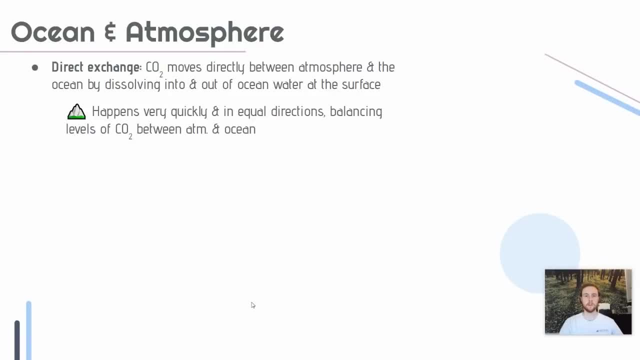 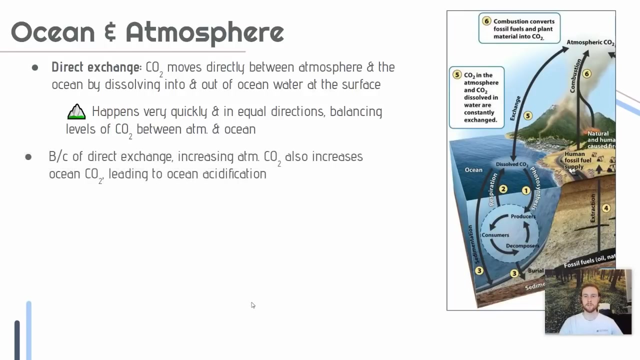 roughly equal directions, So kind of like photosynthesis and cellular respiration. this process results in basically balanced amounts of carbon dioxide in the ocean and the atmosphere. Now, this is a problem as it relates to global climate change, because as we increase the carbon dioxide in the atmosphere, we're also going to increase the carbon dioxide in the atmosphere. So if we increase the carbon dioxide in the atmosphere, we're also going to increase the carbon dioxide in the atmosphere. So if we increase the carbon dioxide in the atmosphere, we're also going to increase the carbon dioxide in the atmosphere. 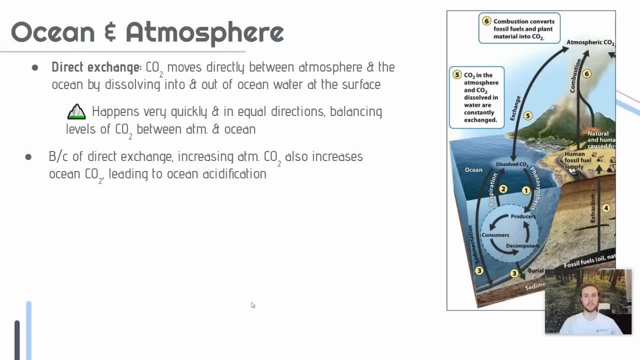 And carbon in the ocean leads to ocean acidification, So the ocean becomes more acidic and that can have consequences for the organisms that live there. If you look at this diagram, look at arrow five. That's going to show this direct exchange where carbon dioxide can move. 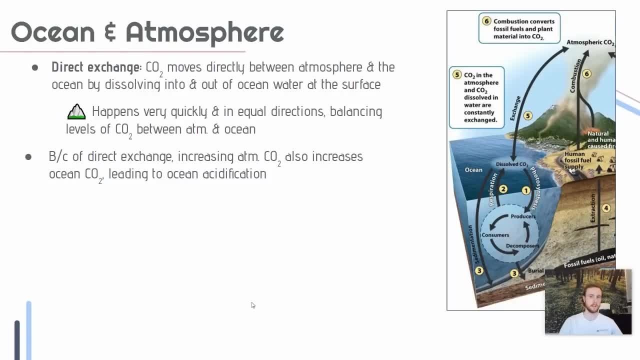 from the atmosphere directly into the ocean and then directly out of the ocean right back into the atmosphere. So again, we call that direct exchange, Now that carbon dioxide in the ocean can be taken up by algae and phytoplankton. 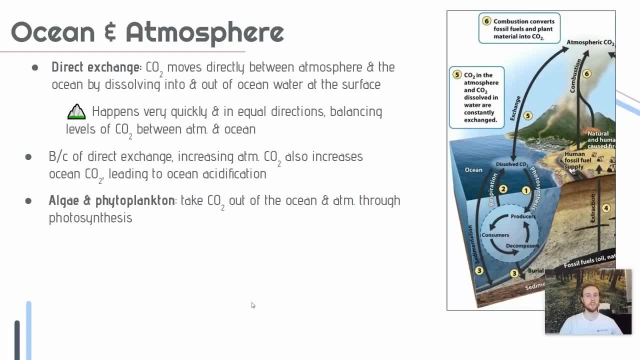 and so they'll take the CO2 and they will convert it into sugars via photosynthesis, So that's one way that the carbon dioxide can be taken out of the ocean. We also have coral reef and other marine organisms that create shells. They're going to take CO2 out of the ocean as well in order to make their shells. 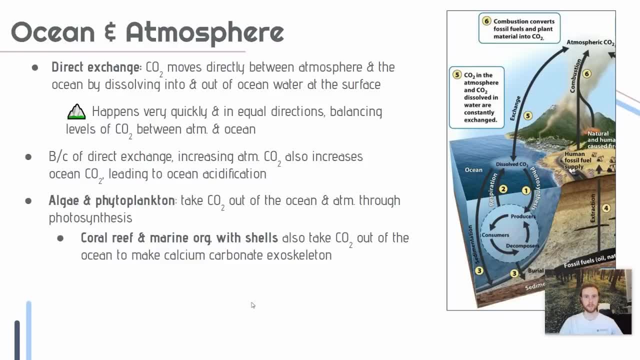 which are made of calcium carbonate. So notice the carbon in calcium carbonate. They're going to have to take that carbon out of the ocean, So they also represent a carbon sink in the ocean so they can remove some of the CO2 added to the ocean by the atmosphere. Sedimentation is the process where, when 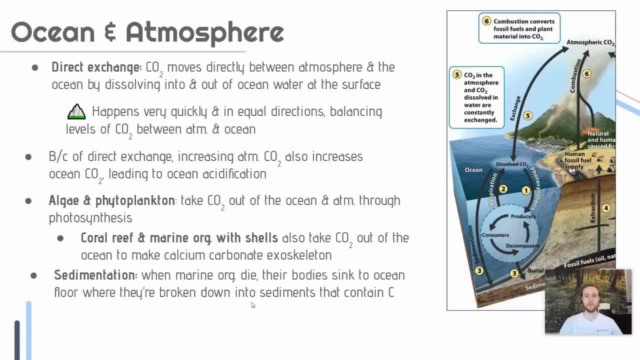 marine organisms die, so coral or fish or shellfish- the remains are going to sink to the bottom of the ocean floor And over time all of the pressure of that water above will smash these organisms down to tiny little pieces that we call sediments. Then burial is a process where 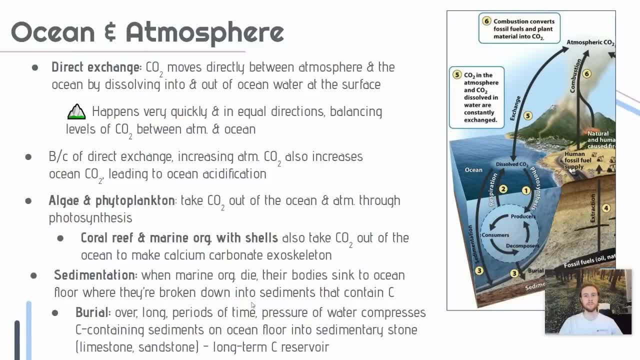 these sediments over long, long periods of time- so thousands, if not millions of years, get all of the pressure of that water in the ocean above them to form sedimentary rock. So these are things like limestone and sandstone, Because they take so long to form. 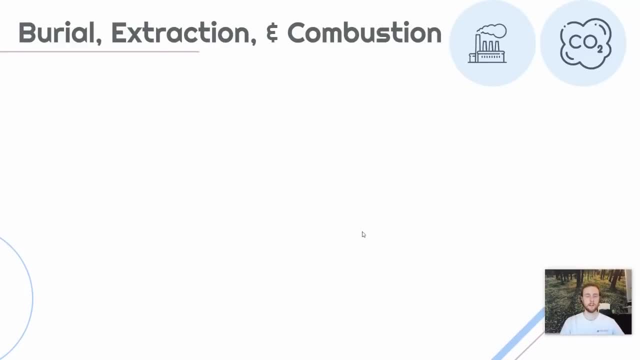 we call them long-term carbon reservoirs. So we'll wrap up our coverage of the carbon cycle today by talking about burial extraction and combustion. So remember that burial is a very slow geological process, meaning it involves rocks that's going to store carbon in underground sinks like sandstone or 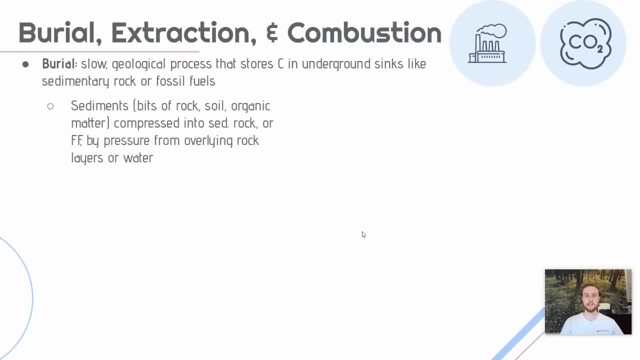 even fossil fuels. So the process is that sediments, so little bits of rock or dead organic matter, will be compressed into sedimentary rock or fossil fuel by the pressure of overlying water or rock layers. So think about little bits of organic matter just getting pressed together over and over. 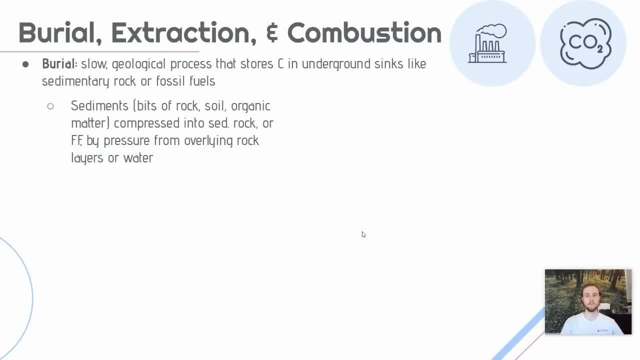 for just millions of years, and eventually they actually form a new substance, which is either a sedimentary rock or, in this case, a fossil fuel. Fossil fuels, coal, oil and natural gas- are also formed through this process of burial and sedimentation. 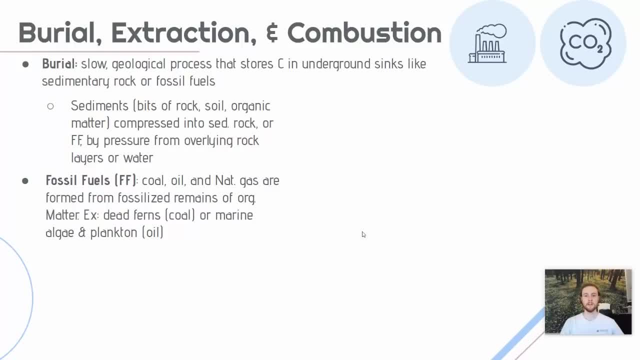 So the fossilized remains of organic matter, especially dead ferns or, if we're talking about oil in the ocean, marine organisms like algae and phytoplankton get compressed by those overlying water or rock layers until they actually compress together to form these fossil fuels.